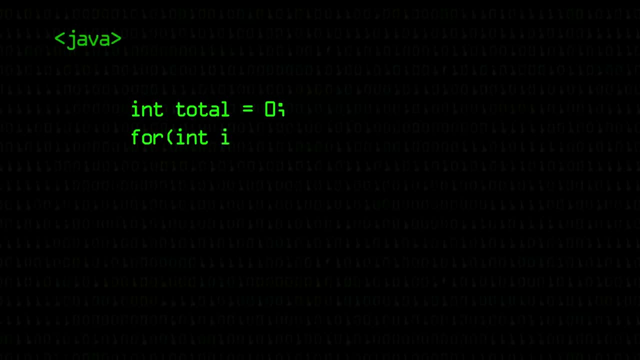 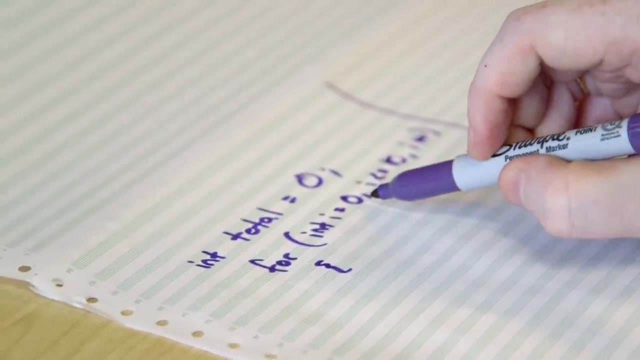 where we say for Sum number, int i equals 0 and i less than or equal to 10, then i plus, plus, And what that means here is we've got this little tracking variable, i, which we initialize to 0. We're going to be repeating this loop as long as it's less than or equal to 10.. 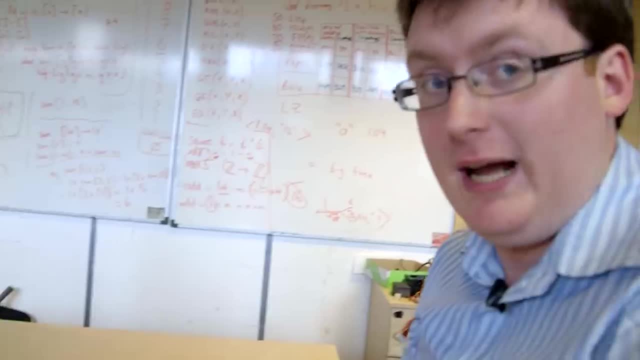 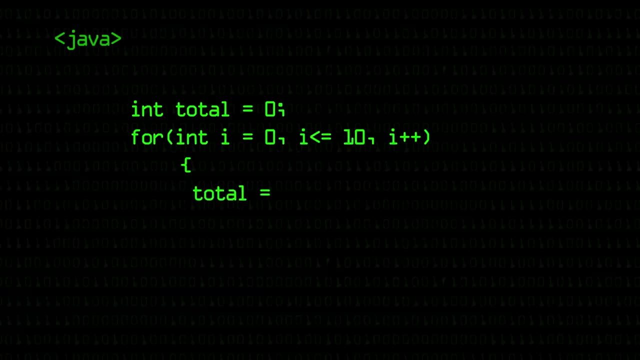 And every time we repeat the loop, we're going to increase i by 1.. We're adding numbers 1 to 10.. So the obvious thing to do is to say: we'll change the variable total to the result, The result of total plus i. 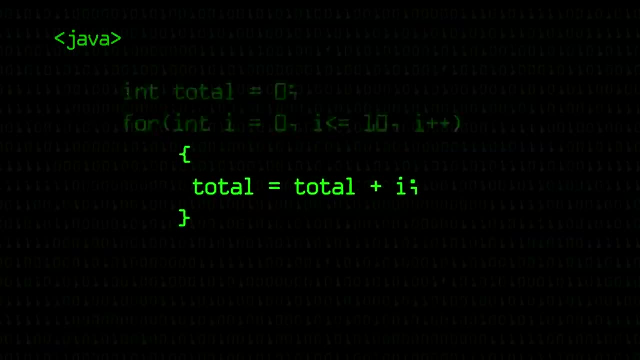 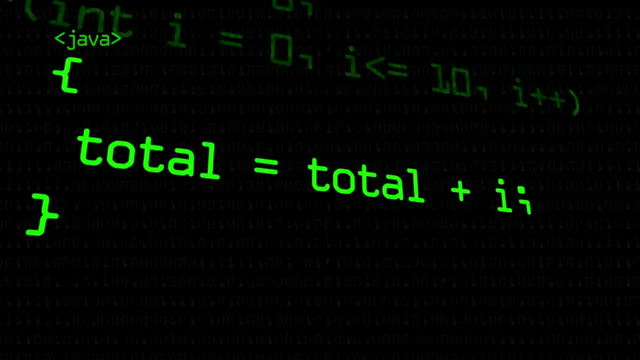 What we have here is we've got an appearance of the equals sign. Some people would look at this and go right. this is clearly the mathematical definition of equals, which means the left hand is equal to the right hand side. That's not the case in Java and other C-like languages. 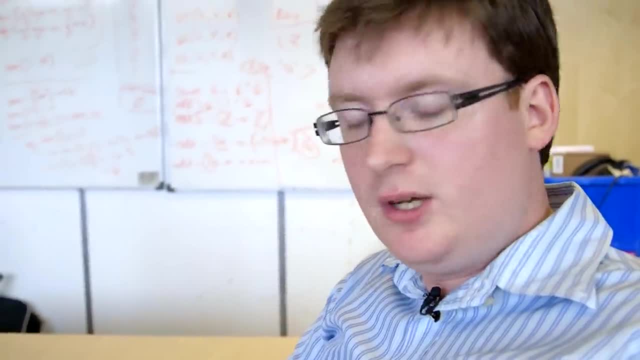 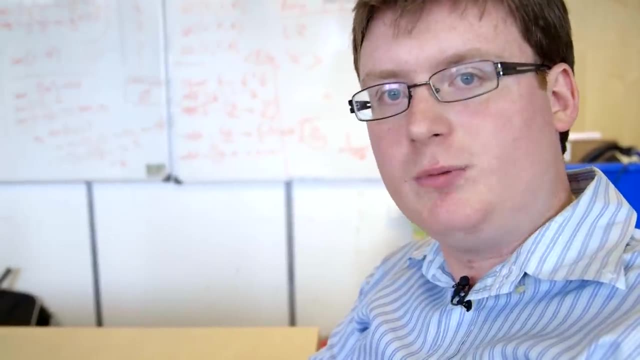 What this single equals actually means is an assignment. We're saying that total is now equal to the previous value of total, and we've edited it in some way In this way: we've added 1 to it. If we were to have a double equals, 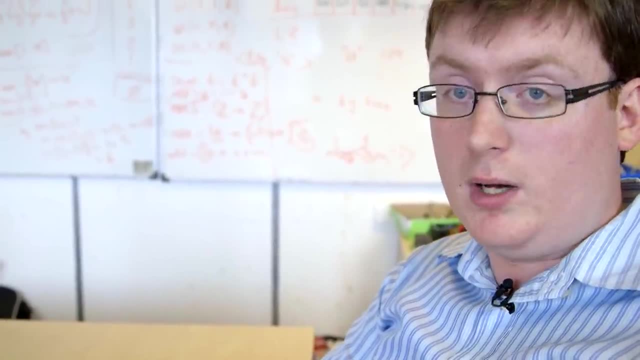 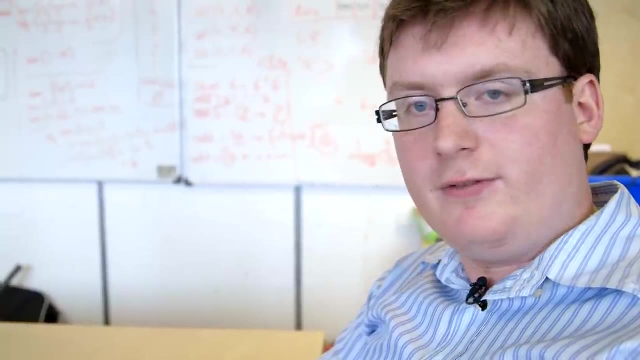 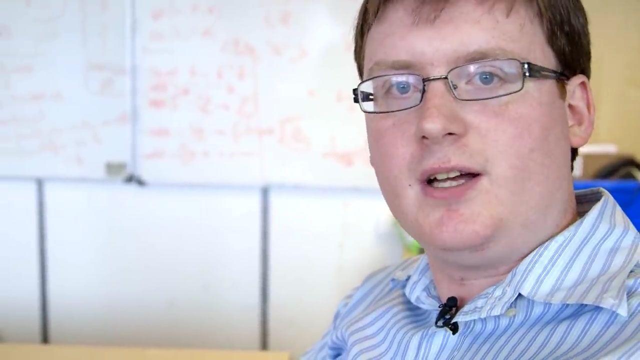 we would be checking for equality, in which case this total equals total plus i would be false in all cases, except for when i was 0. So this kind of statement that involves variables such as total is characteristic of imperative languages where the main method of computation is assignment of values to variables. 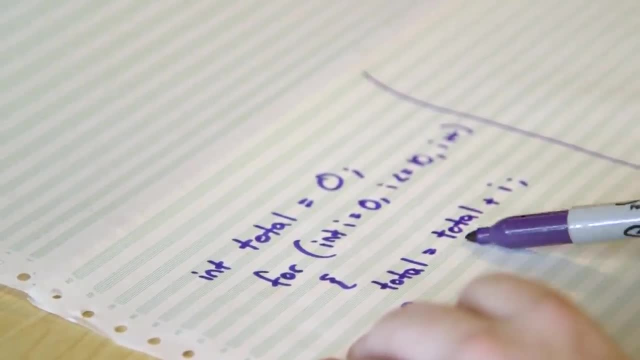 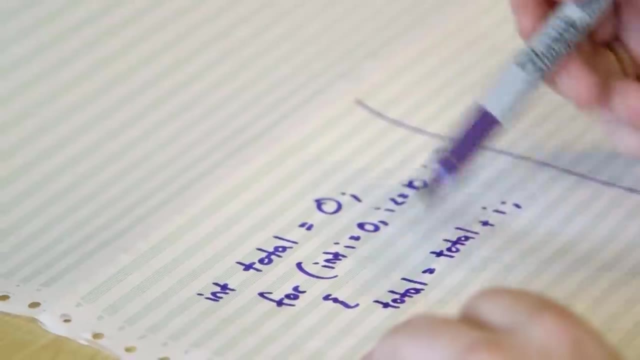 It's going to say: we start with: total is 0. Let me say: if i is 0, total equals 0 plus 0 is 0. Then we go back, We increase i by 1.. So now we say, okay, total is 0 plus 1, which is 1.. 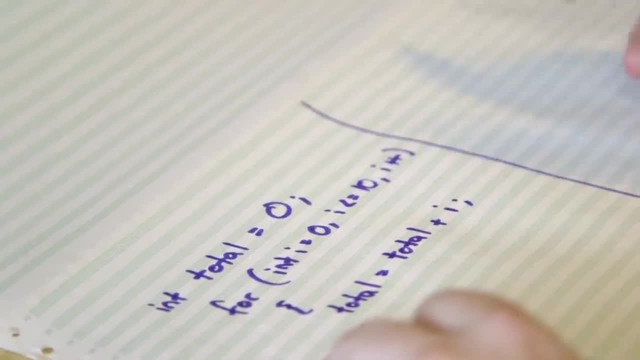 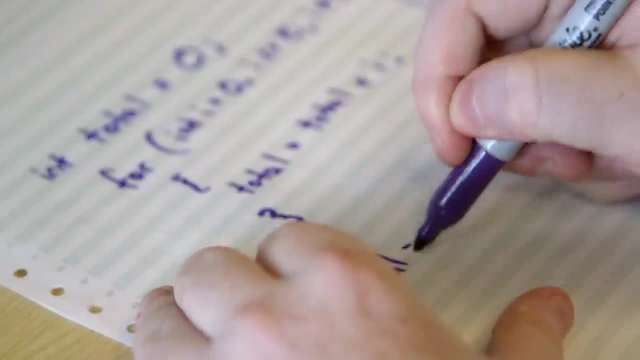 We go back: i is now 2.. Total is 1 plus 2.. It's now 3.. And we repeat: Once we get to the end, then we're done. If we want to call total, then it would just be the result of going 1 plus 2 plus 3 plus da-da-da-da. 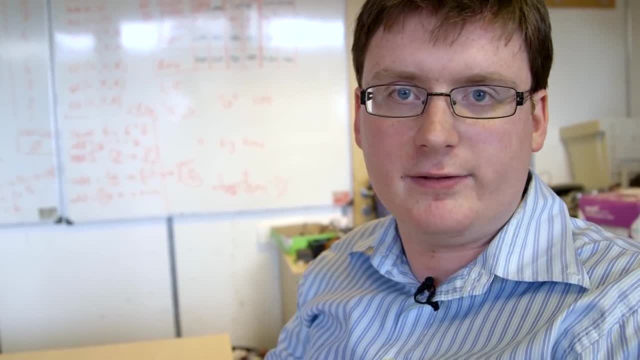 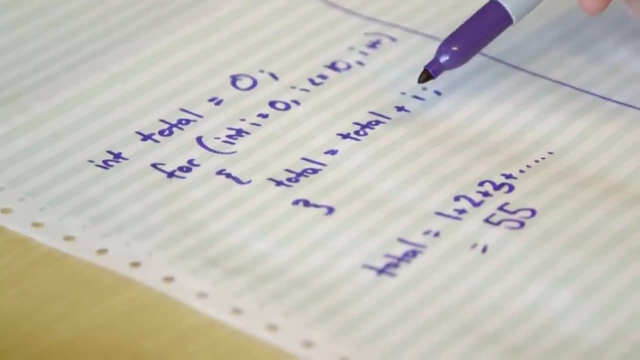 And eventually, at the end of it, we'll have total. if we were to do a call on, it is 55, because that's the sum from 1 to 10.. This is a characteristic of imperative programming, in that we are referring to variables. 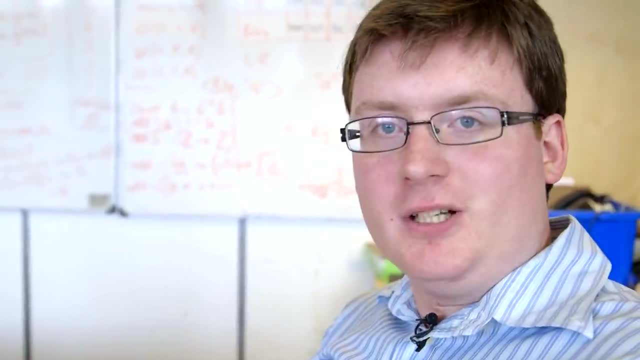 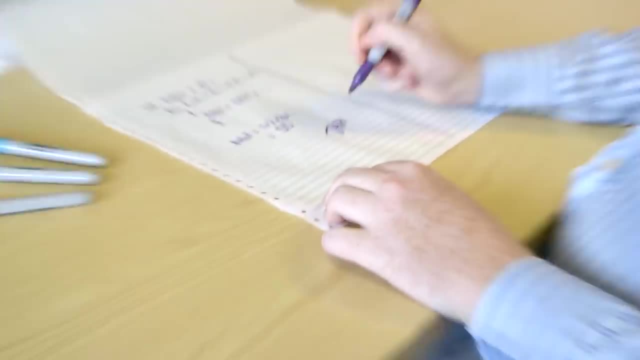 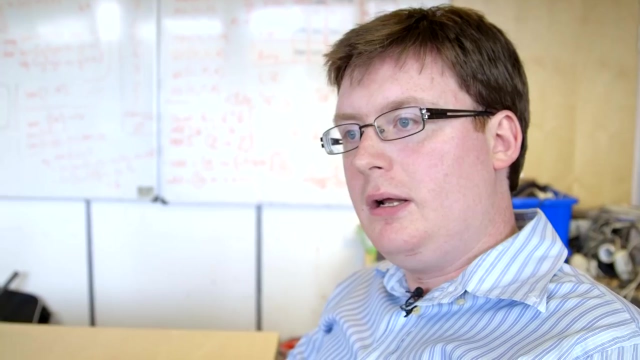 That are defined globally. This is a simple example of adding a couple of numbers up in an imperative language, Namely. this is done in Java. What I'd like to do now, having just spoken about the mathematical definition of equals, move on to another language in which to do this, summing from 1 to 10,. 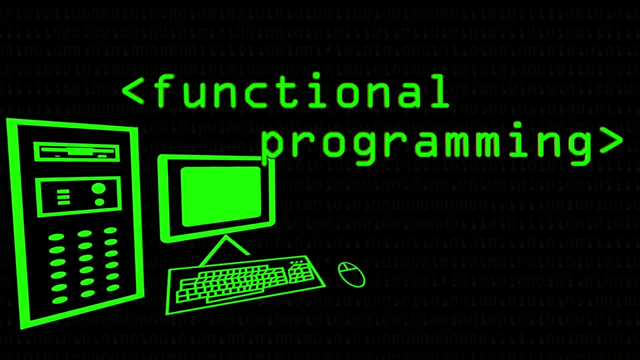 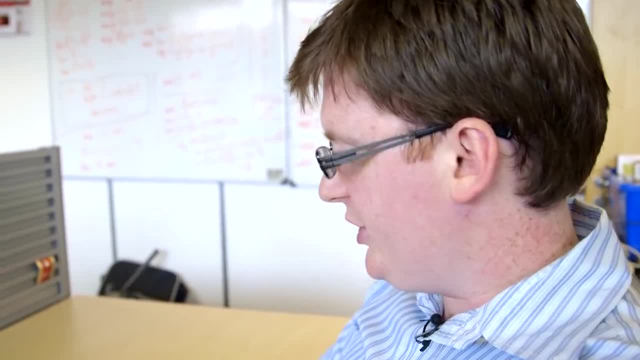 namely Haskell, which is a functional programming language. So the same problem of summing up from 1 to 10 is actually done by what would appear to be magic, By simply going sum 1, 10, done. It's not quite as easy as that. 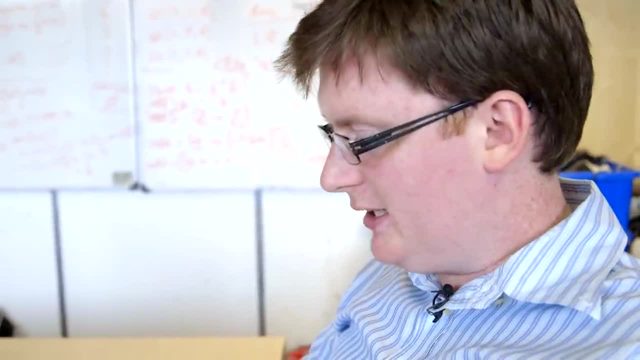 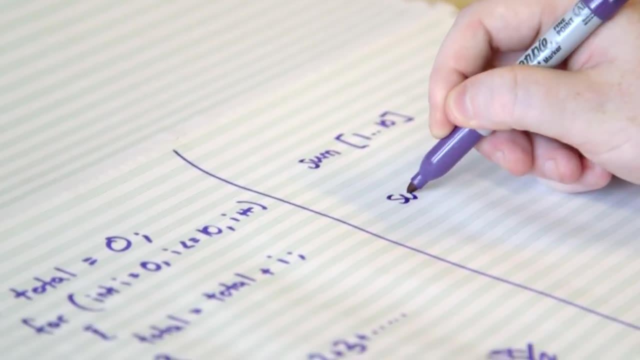 There is a library function in the background that's explaining how sum actually works. The first thing that we need to know about the sum function is what its type is, So we would say that the function sum is the function that takes a list of integers. 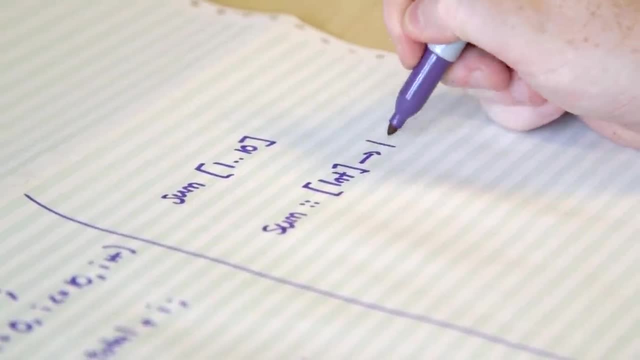 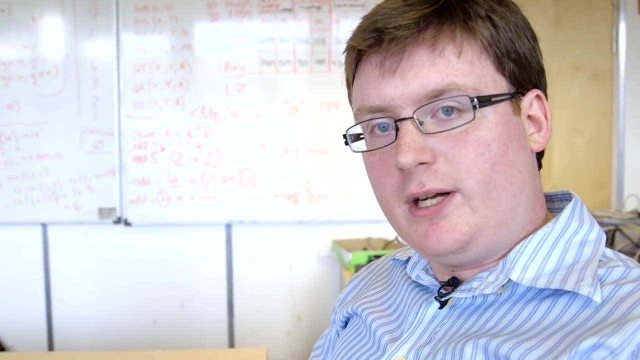 That's the syntax for list, And it returns a single integer, Namely, if we take a list from 1 to 10, we're going to return the sum of them, And what we're going to do now is we're going to define this function in terms of pattern matching. 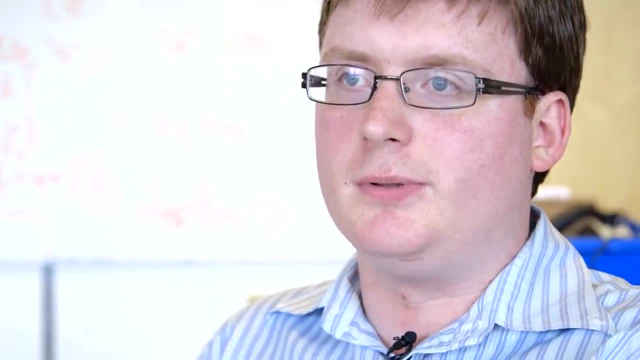 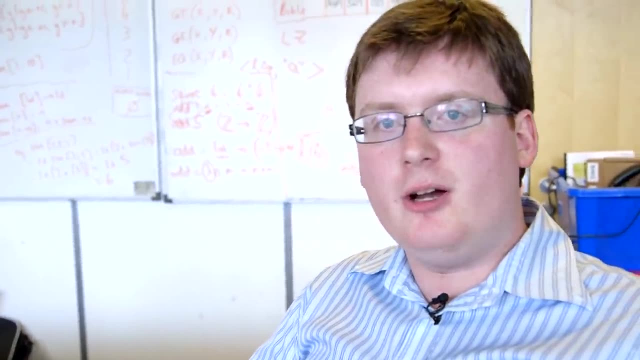 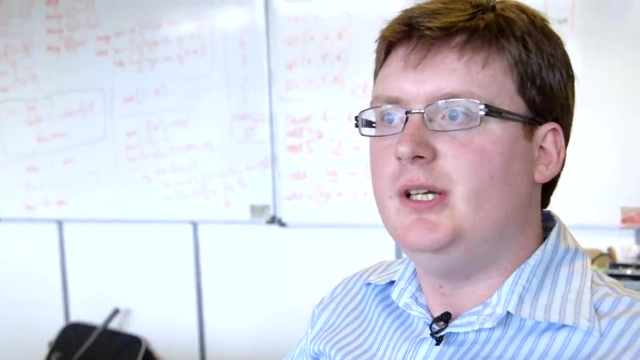 A function can have multiple definitions associated with the value that's given to it. What pattern matching is is a way of deciding which definition of a function to apply in a given case, depending on the structure of the input. So let's say that we are looking at a function that takes lists. 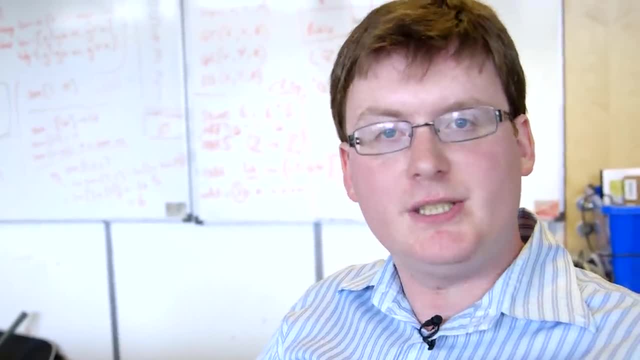 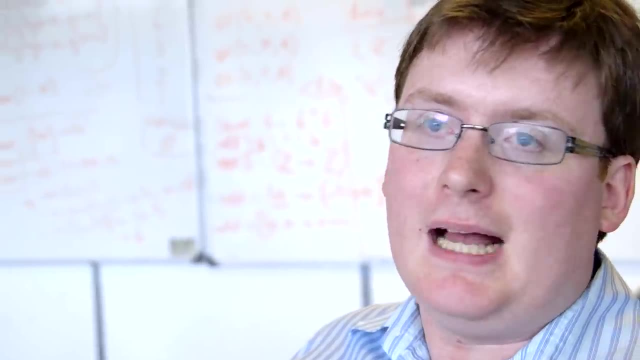 Then that function could be looking at an empty list, It could be looking at a list with one element in it, Or it could be looking at one with more than that. A simpler example, perhaps, is a function that's defined over the booleans. 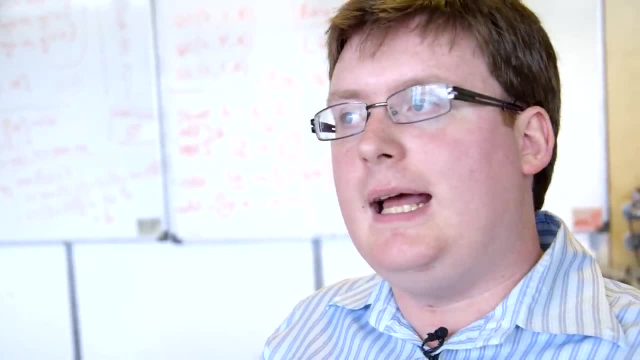 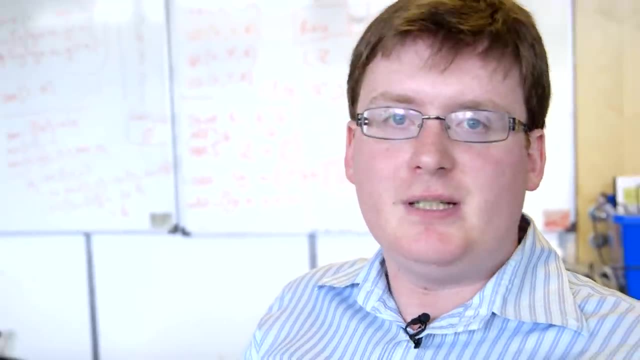 So a boolean value can either be true or false, And a function that's defined over that, the obvious one would be not. So not true is false, not false is true, And if we're using pattern matching, I'm going to take my value. 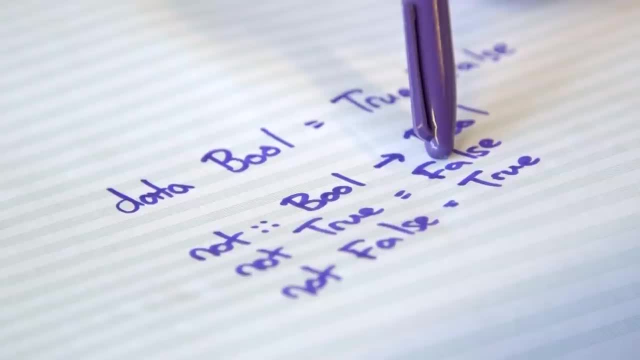 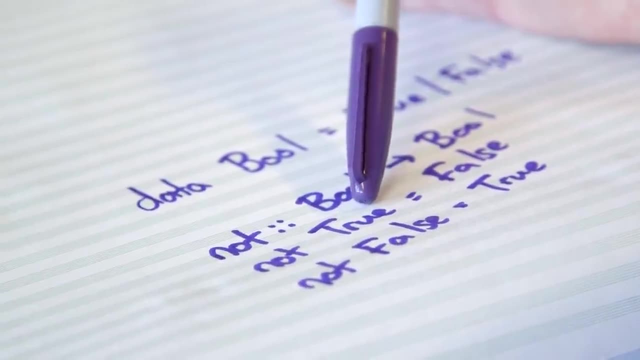 and say: is it true? If the value that I've got is true, then I use the function definition of going to false. If the value that I've got is false, it'll say: I'll look at this first line. Have I got a true? 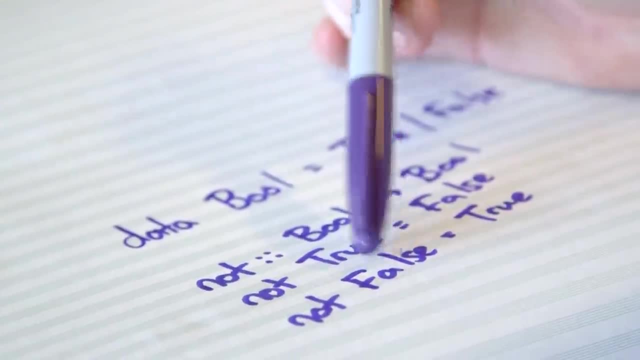 No, I don't, I'll go down to the next one And then I'll say, okay, well, I've got a match there. When you're looking at a function, your inputs, you will try and match from the top. 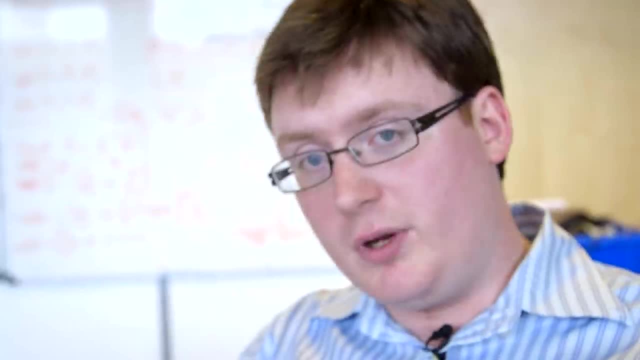 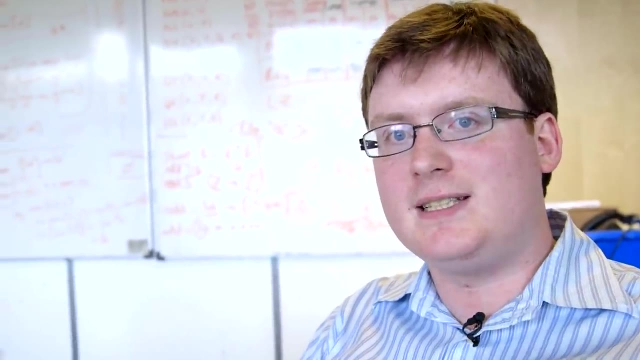 Say: is that the one? I need No Right. look at the next one. Is that the one? I need? No Next one. And it may be the case that you don't have all of the patterns necessary to fully define your function. 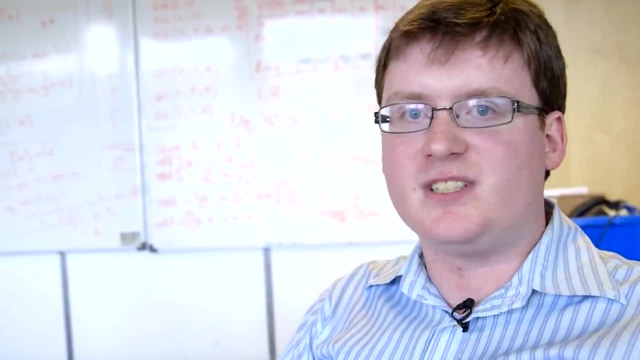 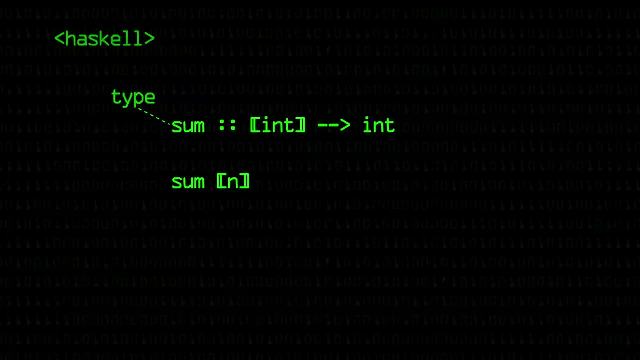 in which case Haskell will give you an error. It'll say non-exhaustive patterns. So if we have this sum of a single number, this is a list of one element. we say that the result of the sum of one number is just that: one number. 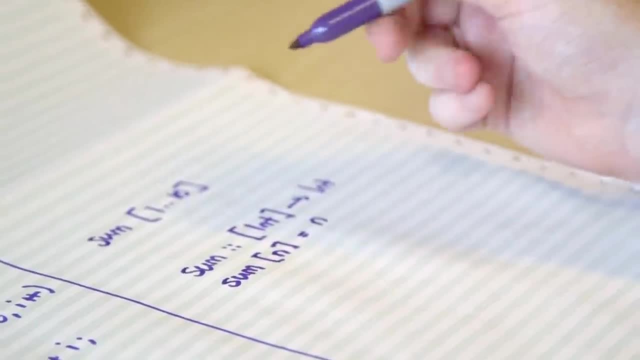 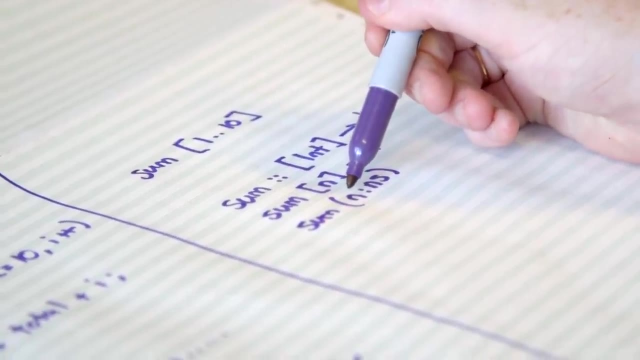 And if we have a list of more than one number, then we would write it like this: sum n- n's. This is just shorthand for saying that the element that's at the front of the list we call n. All the other elements are called n's. 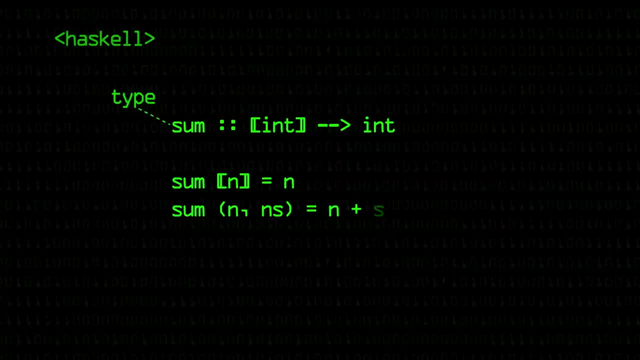 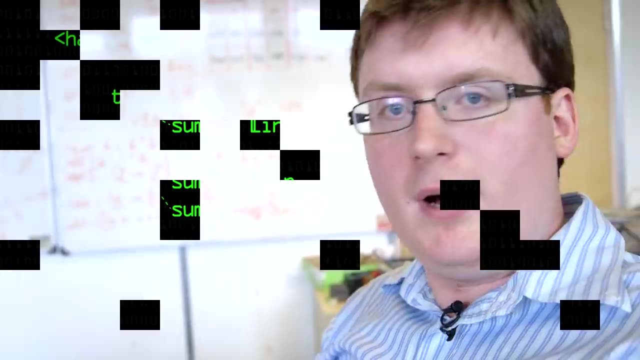 and we would just define that as n plus sum n's. So this function, sum, is defined recursively, that is to say, it's defined in terms of itself. What I might like to do for some people that aren't familiar with functional programming is go through a very quick example. 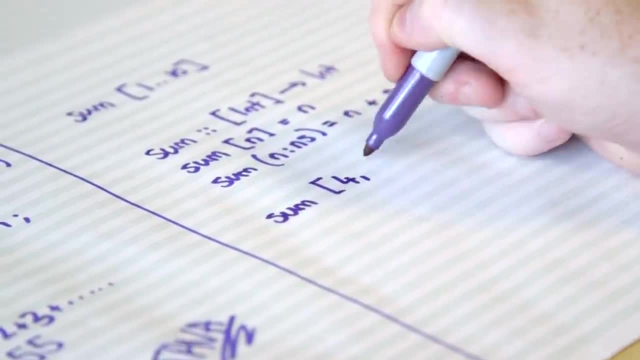 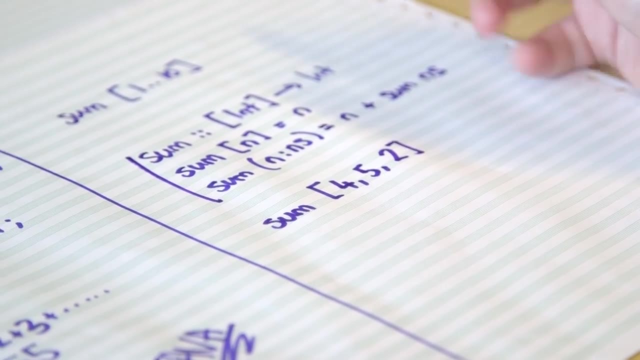 of how the sum function works: Sum of four, five, two. So we can refer to this function here throughout and see how this is equivalent to the Java representation that we've got over here. So what pattern matching involves? we look down and say: 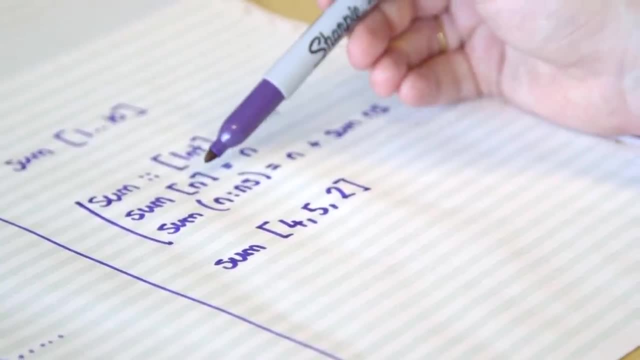 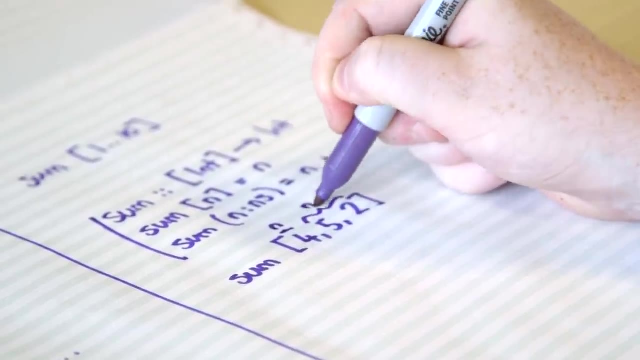 are we looking at a single list? No, we're not. So we can move down to the next pattern and we say: okay, in this instance, this four is the n and this five two is the n's, So this is defined to be. 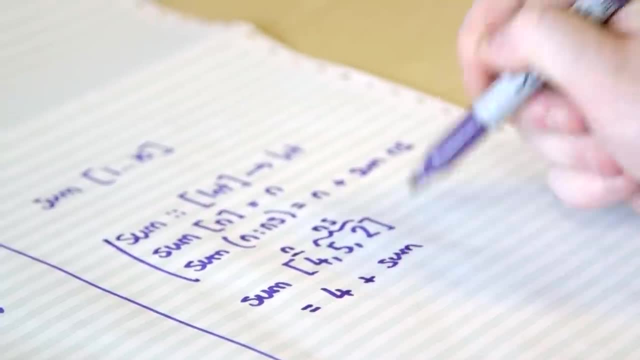 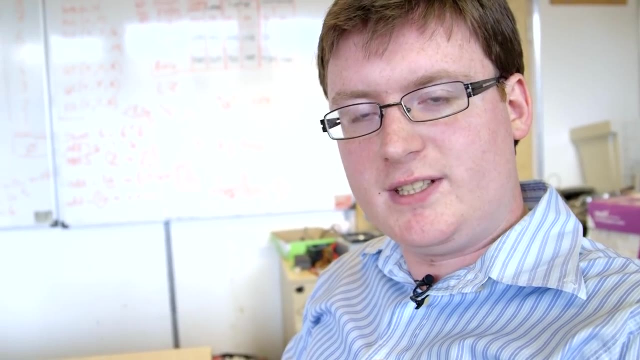 four plus the sum of five and two. Grand Next step: we're going again. sum is defined in terms of itself. We haven't gotten down to base value yet, so we're going to have to carry on. So we do so by saying okay. 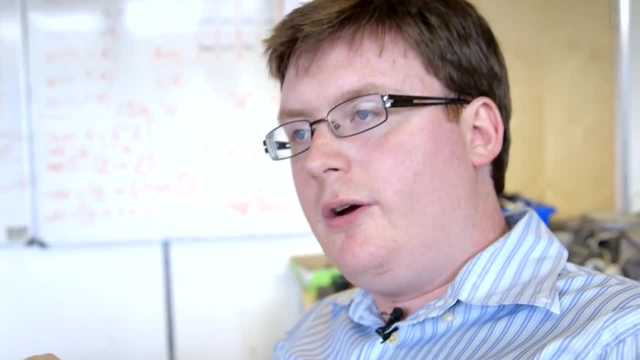 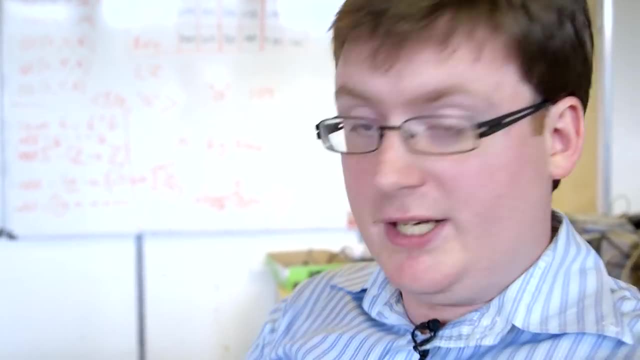 So what do you mean by base value? Okay, So functional programming, the main method of computation for that is applying arguments to functions, as compared with Java, where I said it's assigning values to variables. By here, when I say we've reached a value, 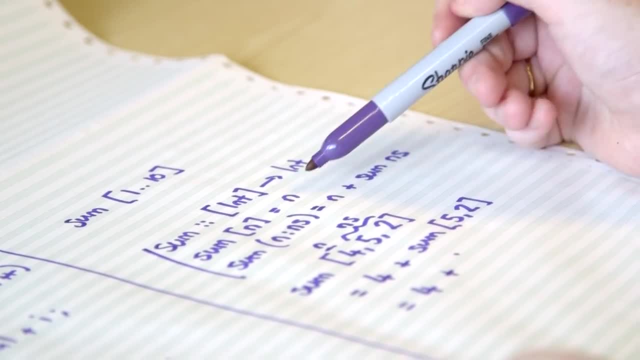 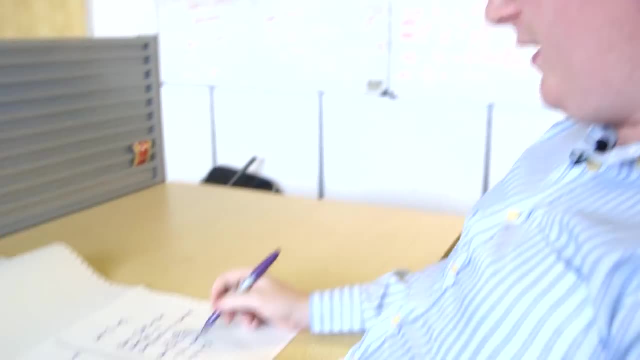 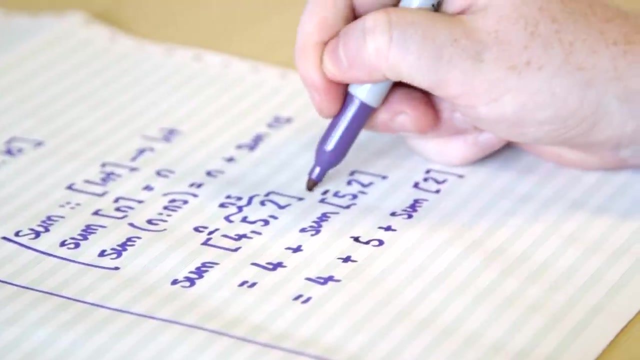 I mean that we've evaluated a singleton and returned n. So to carry on with this evaluation here, what I want to do is to say, okay, that's sum five, two plus sum of two, because in this instance, here this was the n and this was the n's. 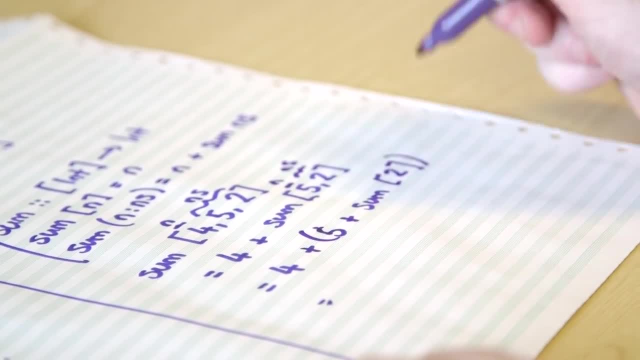 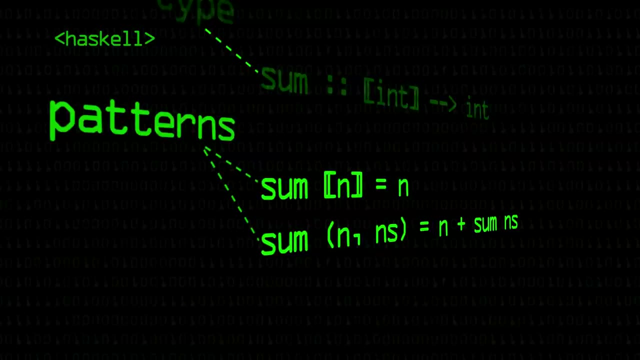 And now I carry on and I say, oh well, if I'm going to be correct, I'm going to bracket that and I'm going to say four plus, five plus. and now I can look and say: pattern matching start from the top. 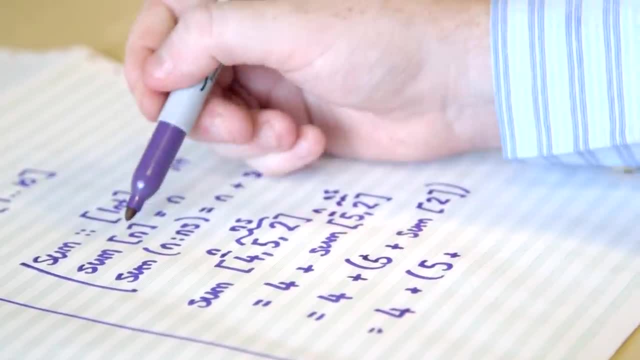 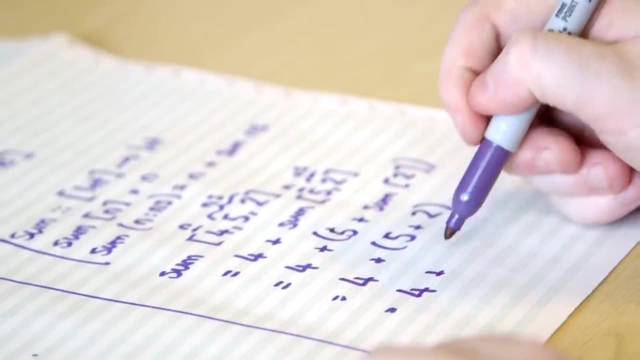 Have I got a singleton list? Yes, I do. So what am I going to return? Just that number two. So now I can start boiling it down. say: well, that's four plus seven equals 11.. So what I've gone through here is just a quick example. 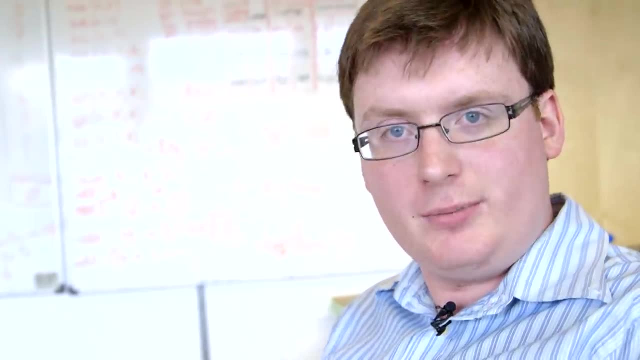 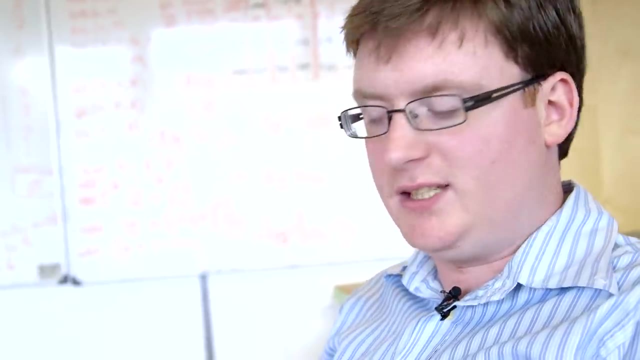 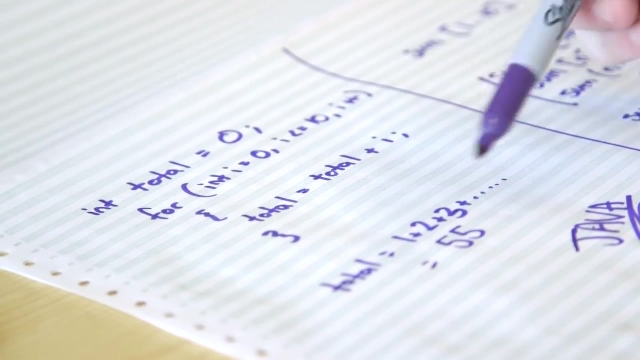 of how a functional programmer would take the approach to the sum function, defining what the sum actually does, as opposed to looking down and doing it in terms of variables, saying, well, track this and add it to this and eventually the result will fall out of it. 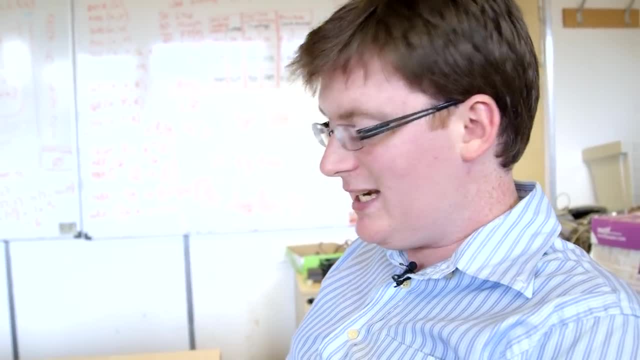 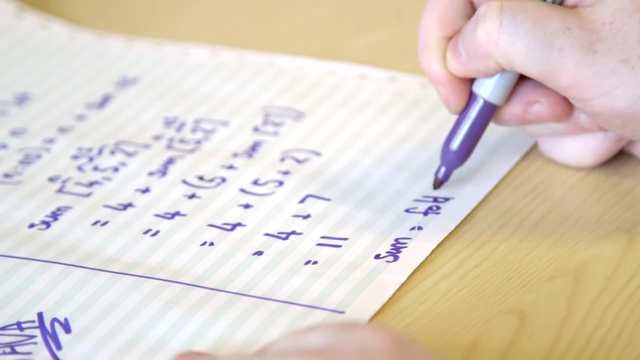 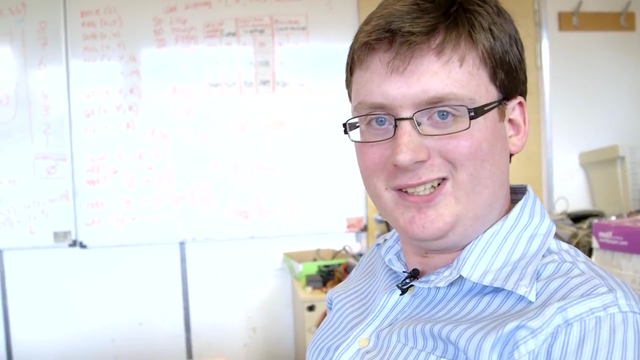 It's probably worth saying, though, that this isn't how sum is defined in the Haskell library. It's actually defined as sum fold L plus zero, but that is dark art that I don't quite want to get into at this video. so 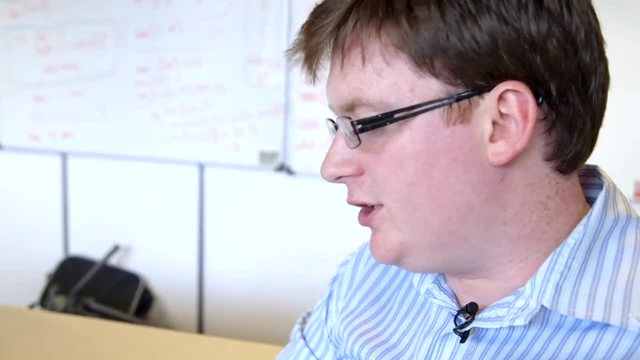 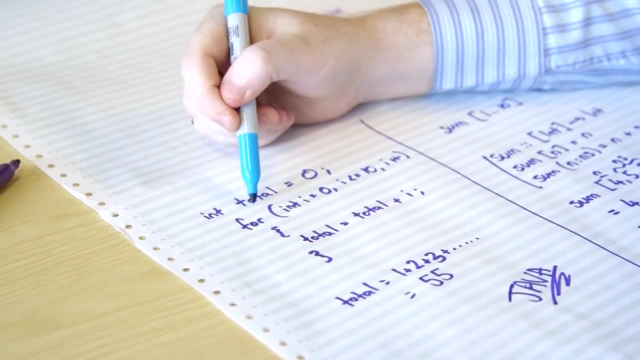 One particularly important thing to take away here, given that I've been contrasting these two, is that in this example here, where I've been summing one to ten in Java, this has revolved somewhat around this variable total, which has been evolving as the for loop progresses. 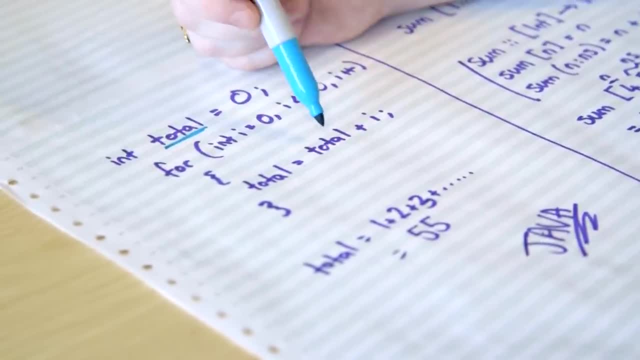 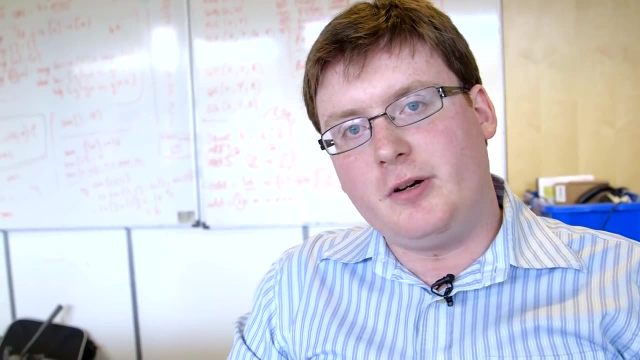 I've been updating this total variable and increasing it to reflect a new value until I get to the end of the for loop. So this is characteristic of imperative programming languages: the fact that I have an external global variable that I can update at will. 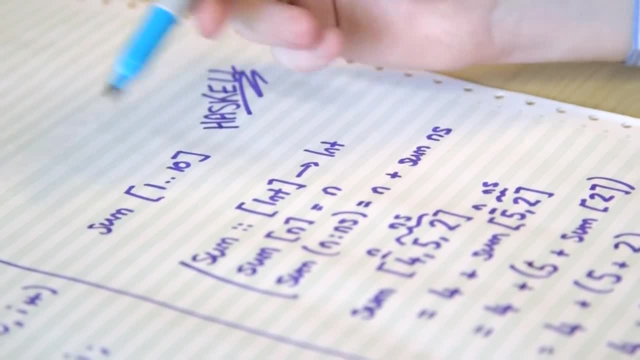 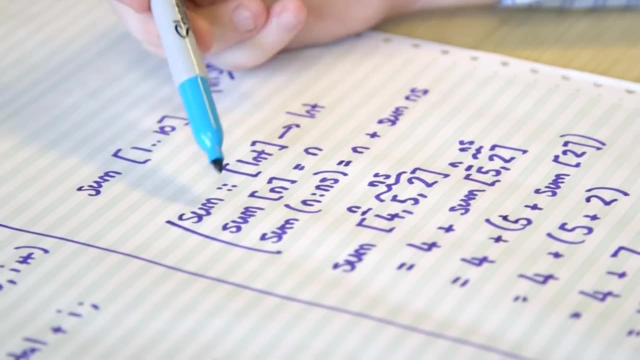 whereas in functional programming, in Haskell, there is no state externally- I'm not calling anything from outside- this sum function, This sum from one to ten, is defined entirely in terms of itself. There is no reference to a total or something that's not explicitly reachable.